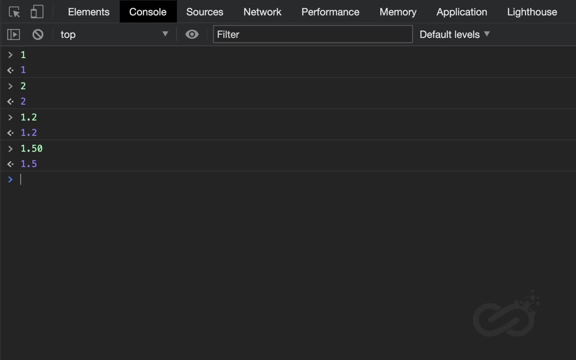 numbers in which we can use the both integer or floating points. and now another data type, that is boolean. what is boolean? the boolean type has only true or false. the boolean has the values yes or no. that means true is yes, correct, false is just false. or in another word, we can say: true is one and 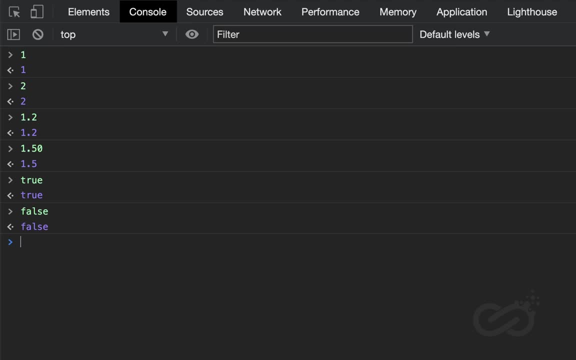 false is zero or true is on and false is off. and there is another data type called null and then undefined. what is null? in null there is no value assigned and in undefined does not have any value assigned to it or initially it is empty. and another primitive data type is that is called 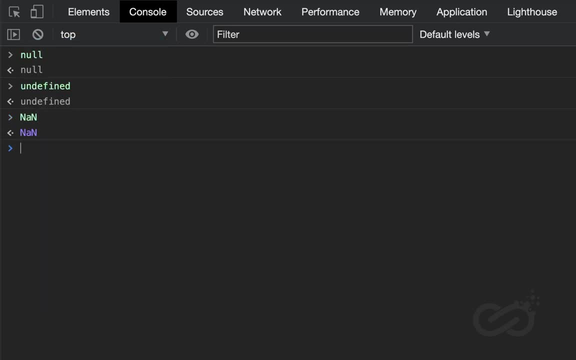 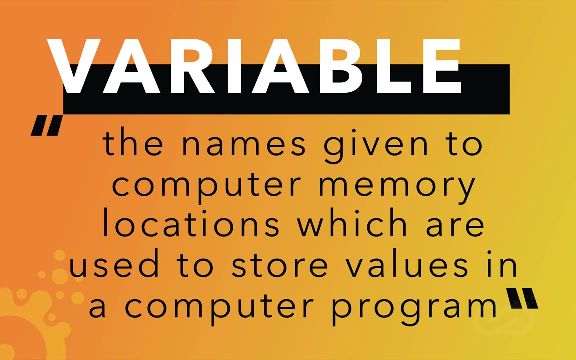 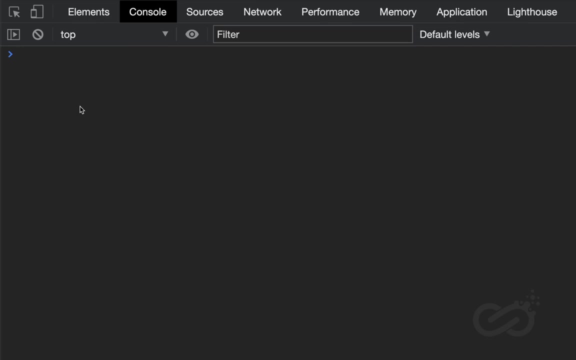 nan. what does nan mean? it means not a number. let's clear out. and what is variable? we need to store values and use the values whenever we need. so how can we do that? we can do that by creating the variable. we can create variable using the key called var. 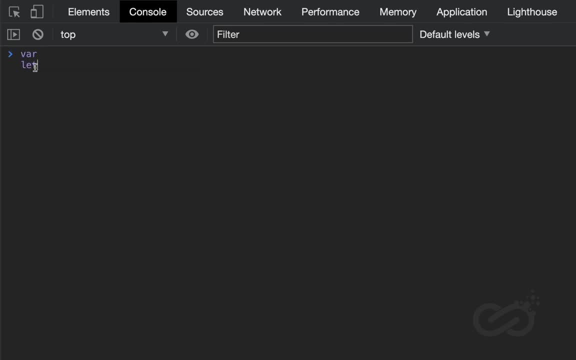 or we can use the let also. let's just clear this now. i will use var. now we have to define our variable name. what is variable variable is just like a box, and we have to level that box with the name, what it will contain or what is containing, something like that. i will just give it a name and then i will just assign. 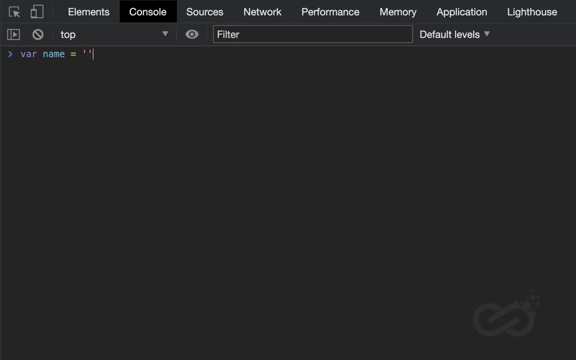 the assign operator that is equal, and then i will give it a string that is hello world. here we have a variable and its name is name and we have assigned the data type string with the value hello world. this assign operator that is equal. we'll take this value and assign it to the 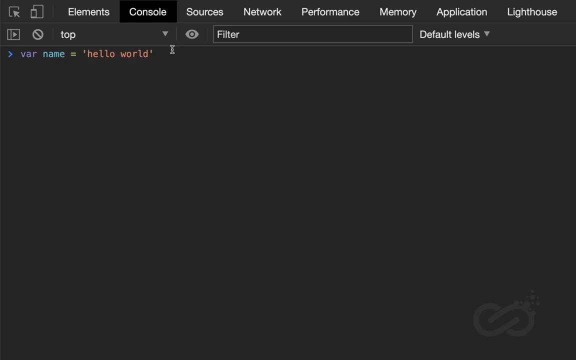 it to the variable with the name that is name. let's just enter, and then i will print out this: how can we print that? just console and then dot log, and then we will use the variable name- that is name- and then enter. here we can see the hello world that we have assigned. now let's create a.